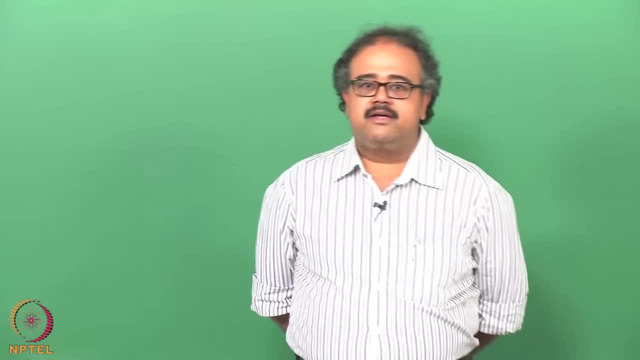 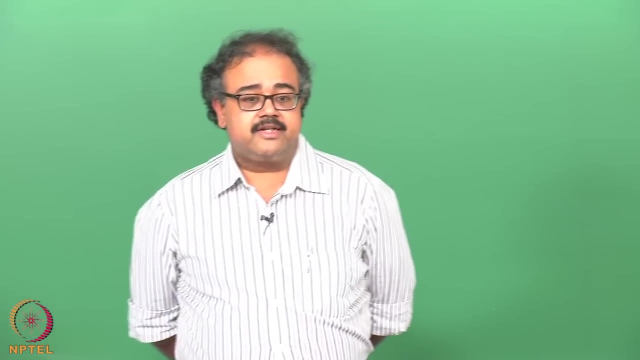 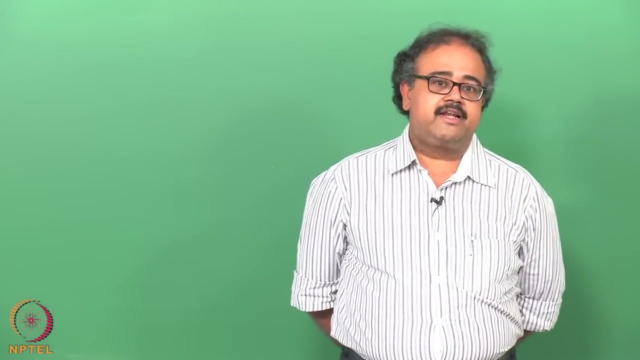 actually far away from all the other points in the data set to be considered as what are known as outliers. So when you do clustering there are two things. So one is you are interested in finding cohesive groups of points and second is you are also interested in finding data points that do not confirm to the patterns in the input and 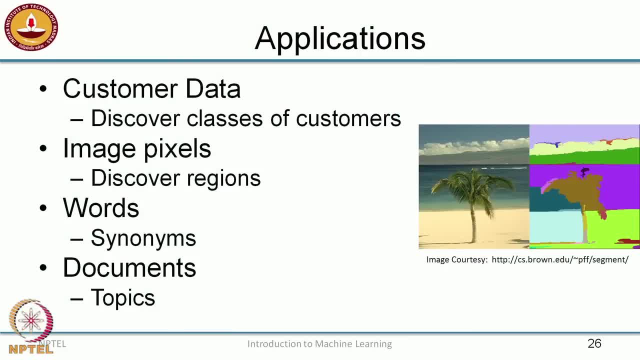 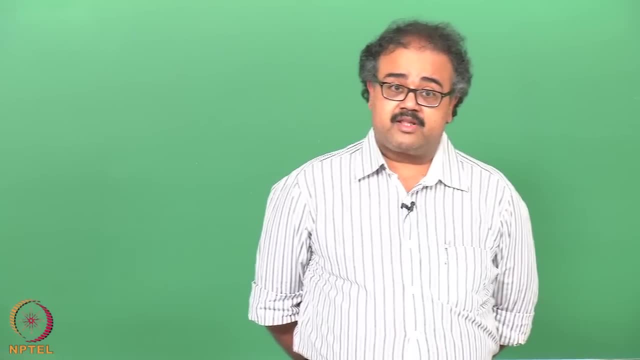 these are known as outliers right, and so many, many different ways of which you can accomplish clustering- and we will look at a few in the course- and the applications are numerous right, so here are a few representative ones. So one thing is to look at customer data right and try to discover classes of customers. you 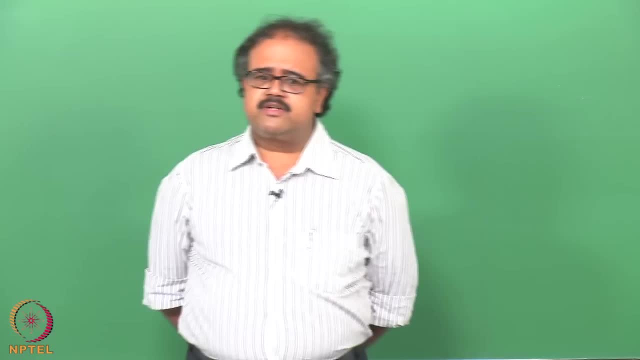 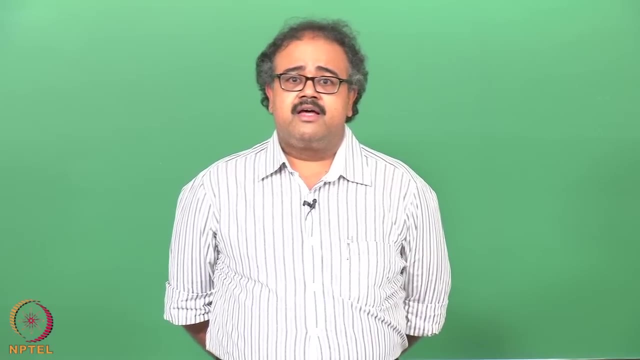 know there are. so earlier we looked at in the supervised learning case we looked at whether a customer will buy a computer or will not buy a computer. as opposed to that, we could just take all the customer data that you have and try to just group them into different. 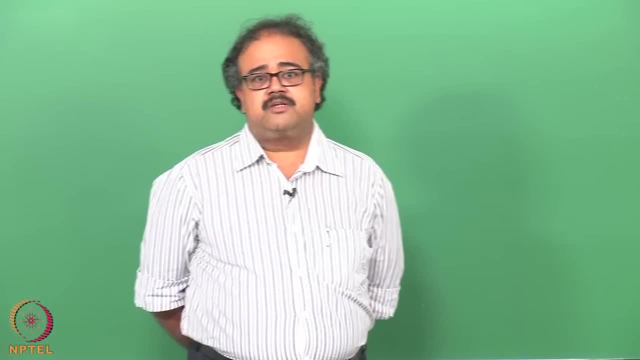 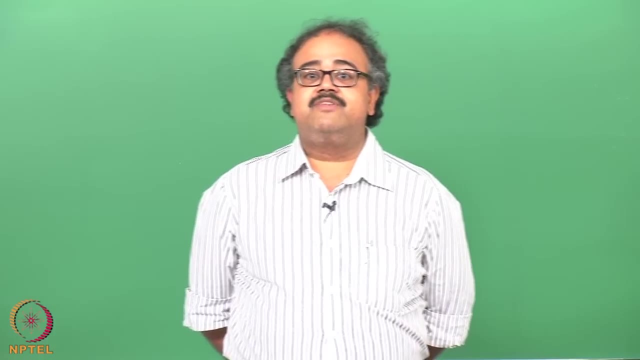 kinds of customers who come to your shop. and then you could do some kind of targeted promotions at different classes of customers, right, and this need not necessarily come with labels, you know, I am not going to tell you that. okay, this customer is class 1, that customer is: 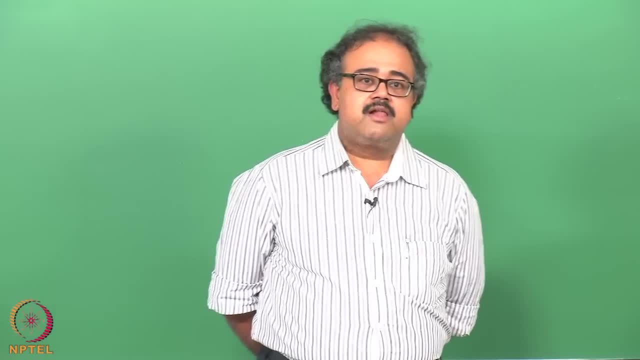 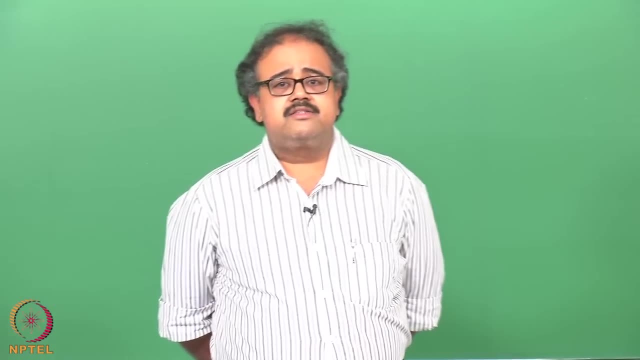 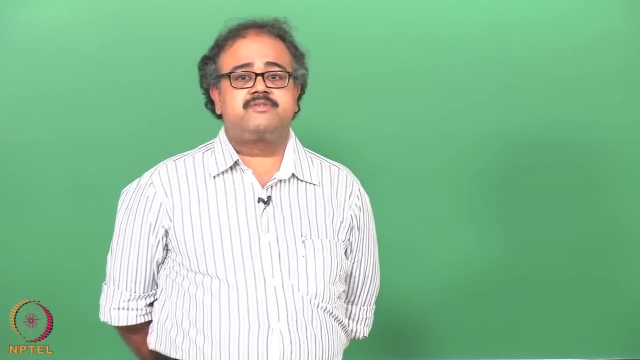 class 2, you are just going to find out which of the customers are more similar with each other. right, And as a second application which I have illustrated Here, is that I could do clustering on image pixels so that you could discover different regions in the image and then you could do some segmentation based on that different 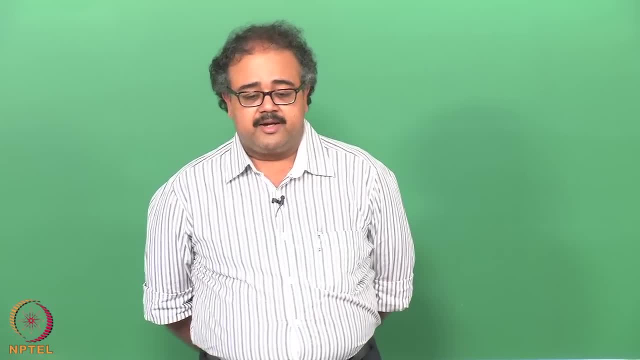 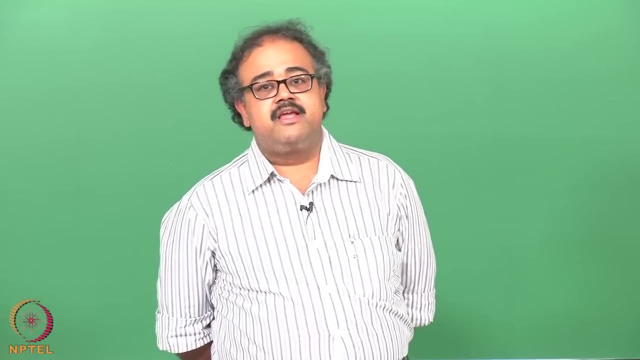 region. so, for example, here it have a picture of a picture of a beach scene and then you are able to figure out the clouds and the sand and the sea and the tree from the image. so that allows you to make more sense out of the image, right? or you could do clustering. 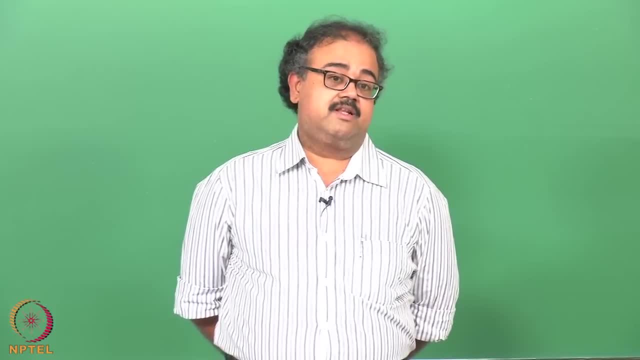 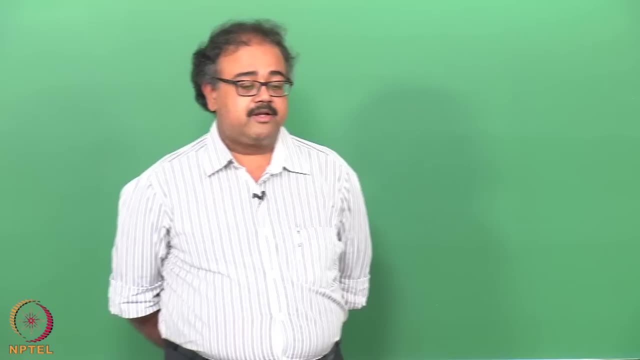 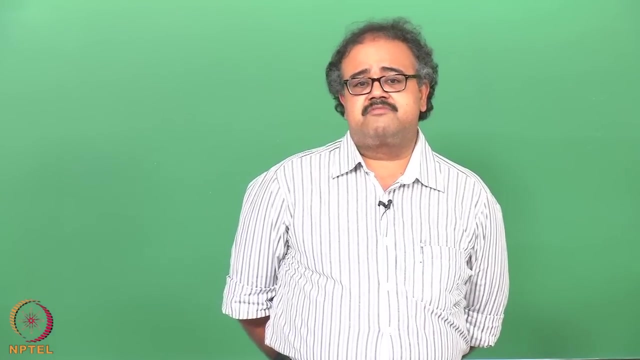 on word usages: right, And you could discover synonyms. and you could also do clustering on documents: right, and depending on which kind of documents are similar to each other, right. if I give you a collection of, say, 100,000 documents, I might be able to figure out what are the different topics that 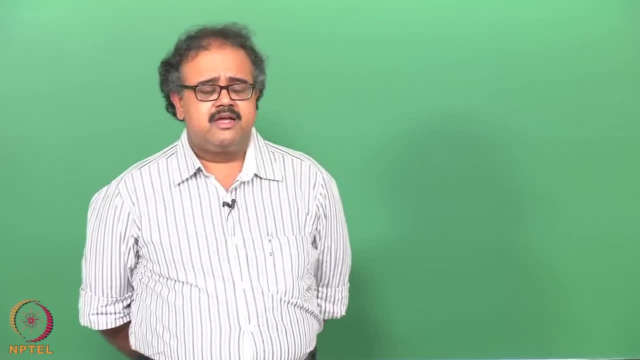 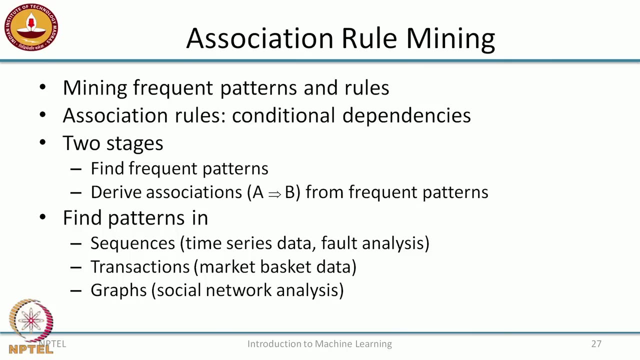 are discussed in this collection of documents and many, many ways in which you can use clustering rule mining, And so I should give you a side about this. Thank you very much. The usage of the word mining here: So many of you might have heard of the term data mining and, more often than not, the purported 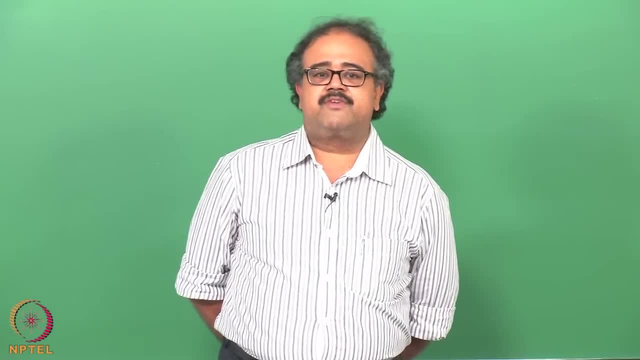 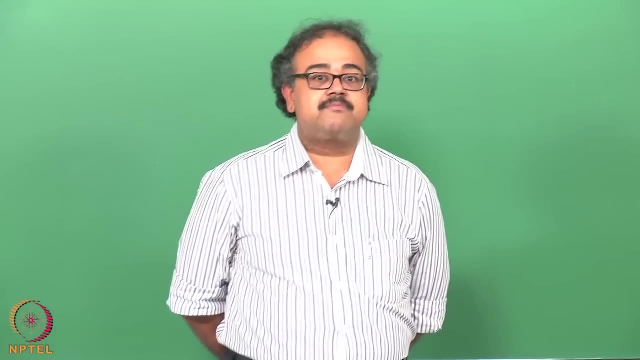 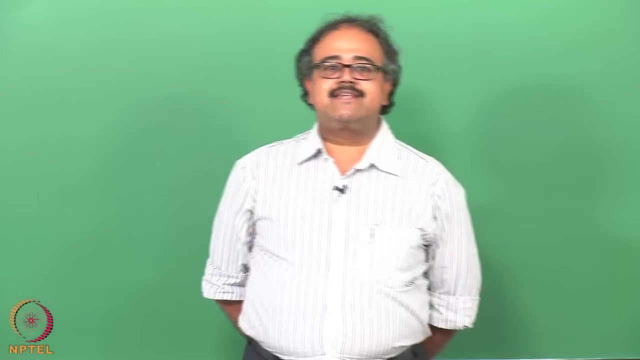 data mining tasks are essentially machine learning problems. right, so it could be classification, regression and so on, so forth. and the first problem that was essentially introduced as a mining problem and not as a learning problem was the one of mining frequent patterns and associations, And that is one of the reasons I call this association. 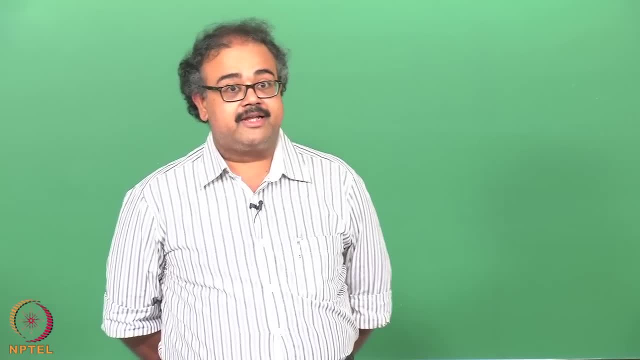 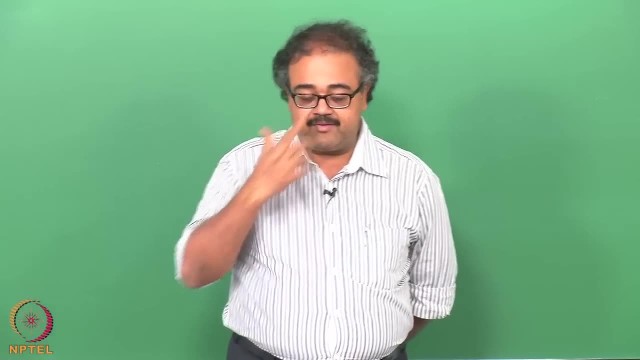 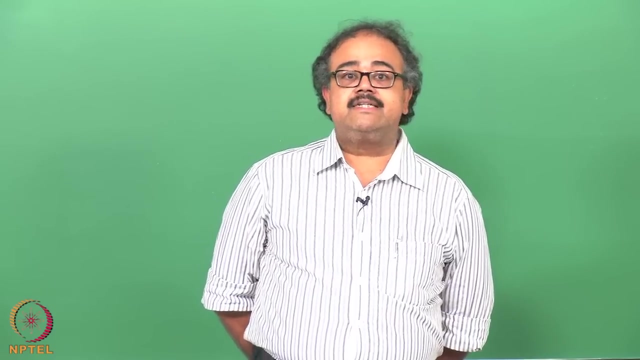 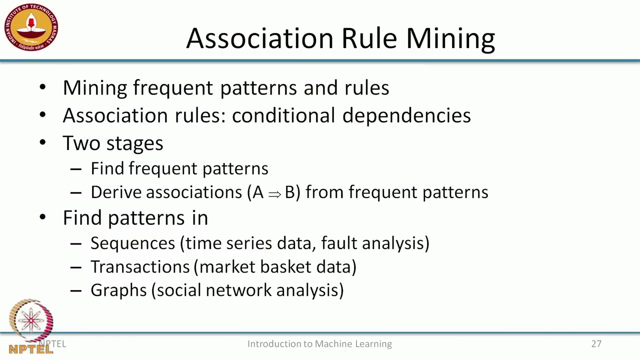 As association rule mining, as opposed to association rule learning, just to keep the historic connection intact, right. So in association rule mining we are interested in finding frequent patterns that occur in the input data, and then we are looking at conditional dependencies among these patterns. right, And so, for example, if A and B occur together often, right. then I could say something like: 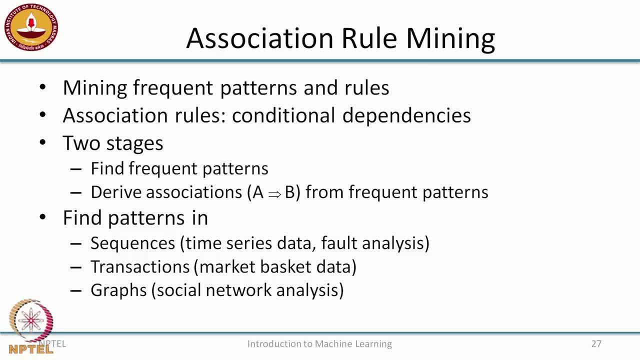 if A happens, then B will happen. Let us see, Let us suppose that. so you have customers that are coming to your shop and whenever customer A visits your shop, customer B also tags along with him, right? So the next time you find customer A somewhere in the shop, so you can know that customer. 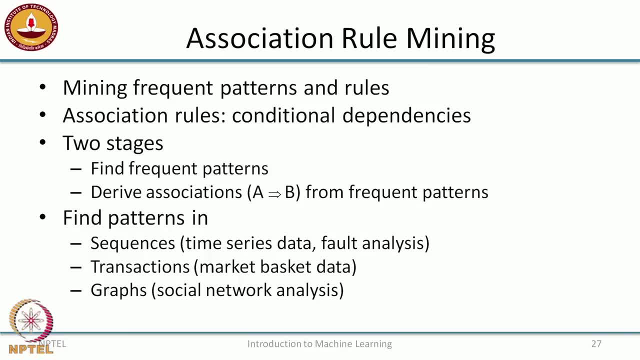 B is already there in the shop along with A, Or, with very high confidence, you could say that B is also in the shop at somewhere else, maybe not with A, but somewhere else in the shop, right? So these are the kinds of rules that we are looking at. 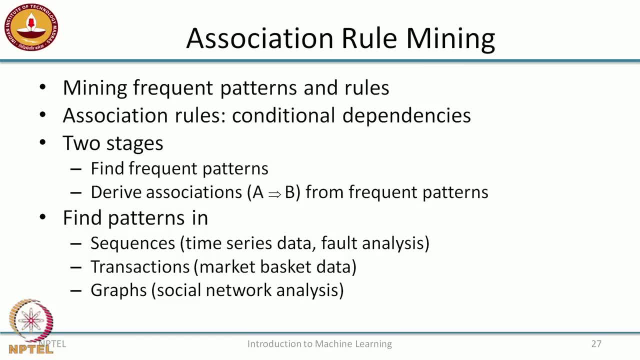 association rules, which are conditional dependencies. if a has come, then b is also there right, and so the association rule mining process usually goes in two stages. so the first thing is we find all frequent patterns. so a, a happens often. so a is a customer that comes to my store often. 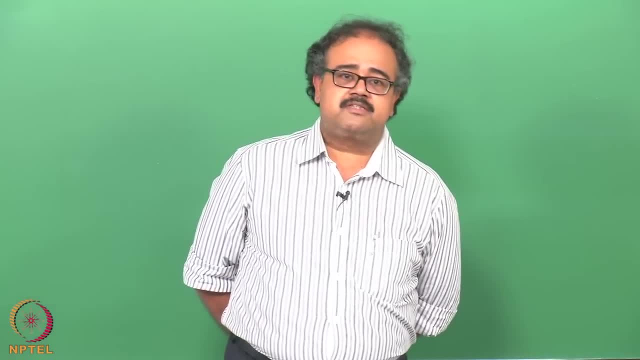 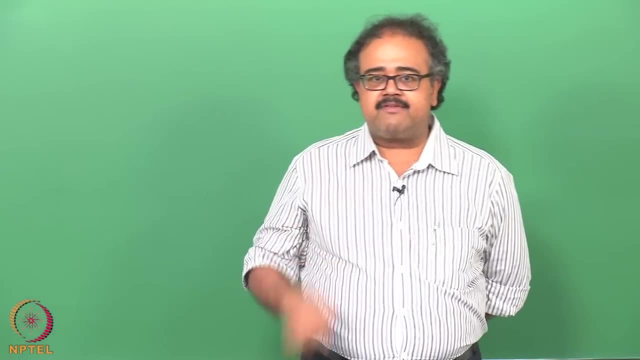 right. and then i find that a and b are pairs of customers that come to my store often. so if i once i have that right- a comes to my store often and a and b comes to my store often- then i can derive associations from this kind, this frequent patterns, right, and so you could do this in a variety of 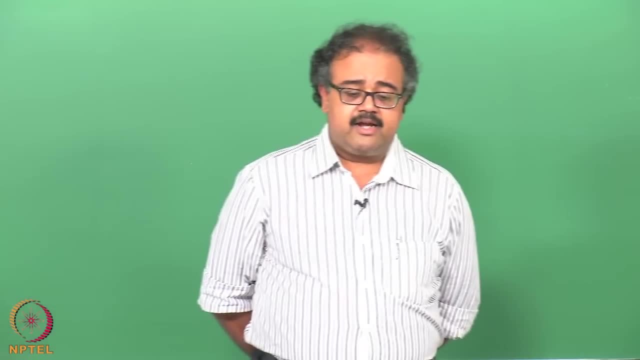 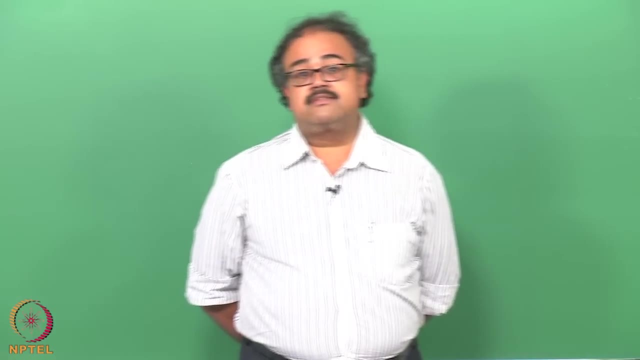 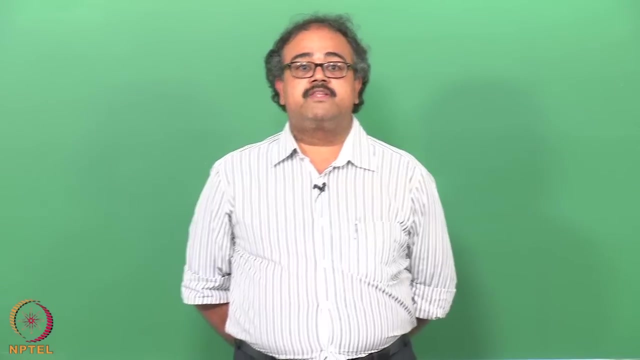 different settings. you could find sequences in time series data right and where you could look at triggers for certain events. or you could look at fault analysis right by looking at a sequence of events that happened and you can figure out which event occurs more often with the fault. 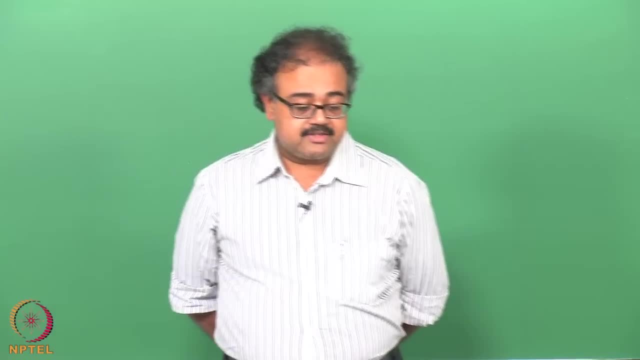 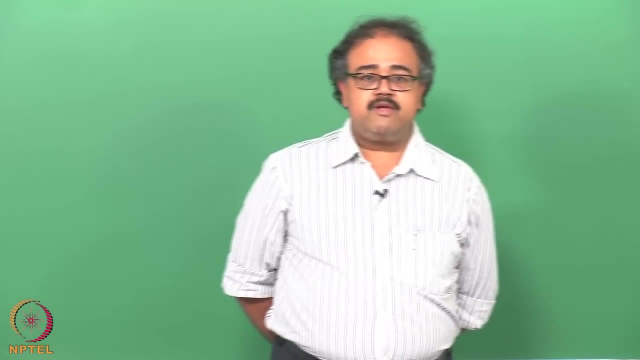 right, or you could look at transactions data. which is the most popular example given here is what is called market basket data. so you go to a shop and you buy a bunch of things together and you put them in your basket. so what is there in your basket, right? so this forms the transaction. so 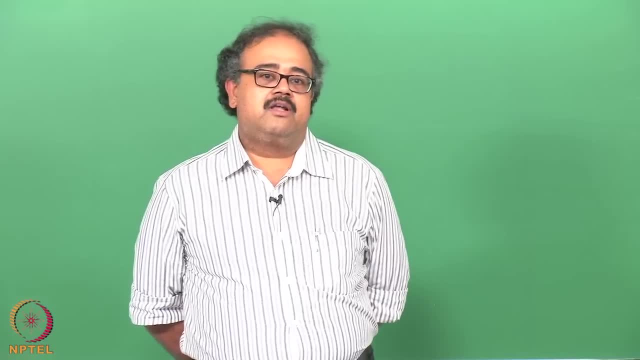 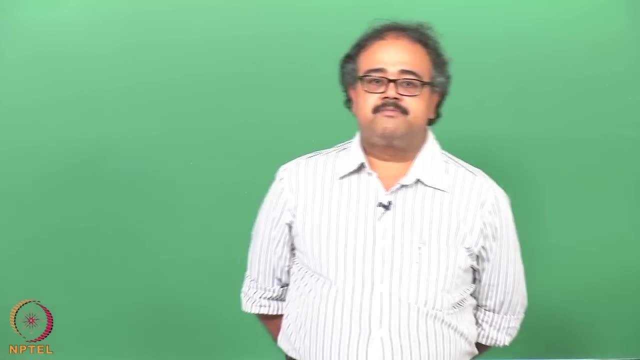 you buy, say, eggs, milk and bread, and so all of these go together in your basket and then you can find out what are the frequently occurring patterns in this purchase data and then you can make rules of the market right. so this is the most popular example given. here is what is called 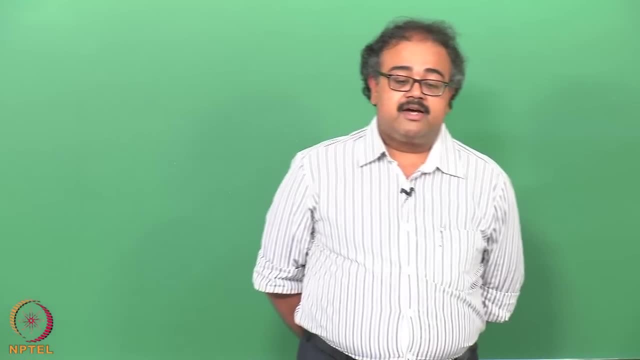 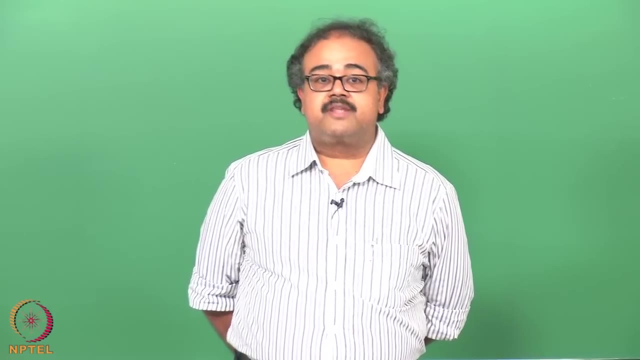 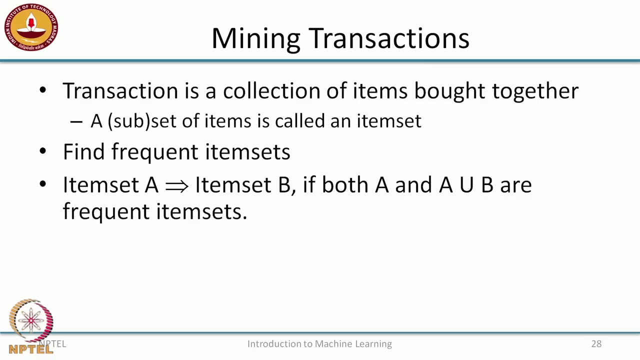 market basket data. so what are the frequently occurring patterns in this purchase data and those or you could look at finding patterns in graphs. that's typically used in social network analysis. so which kind of interactions among entities happen often, right, so that is a that's another question that's worth looking at. right so the most popular 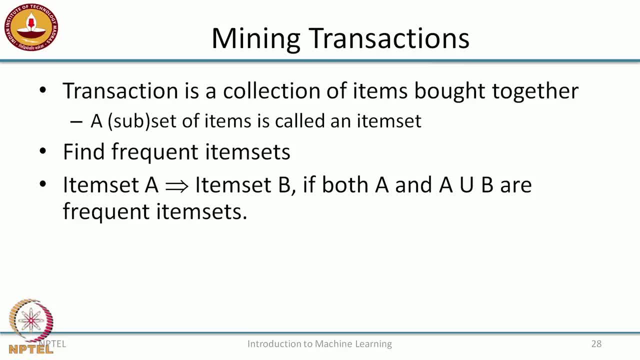 thing here is mining transactions, so the most popular application here is mining transactions and, as i mentioned earlier, transaction is a collection of items that are bought together, right, and so that's what we are looking at right. so the most popular thing here is mining transactions. So here is a little bit of terminology, and a set or a subset of items is often called. 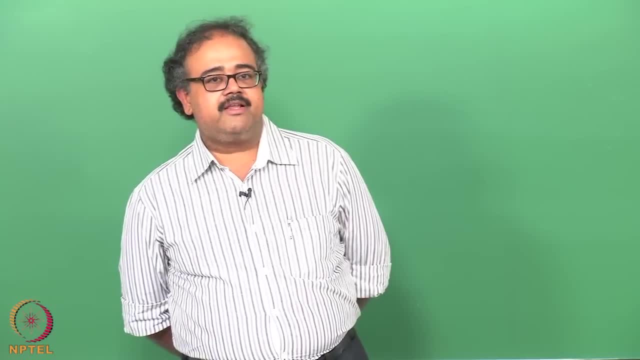 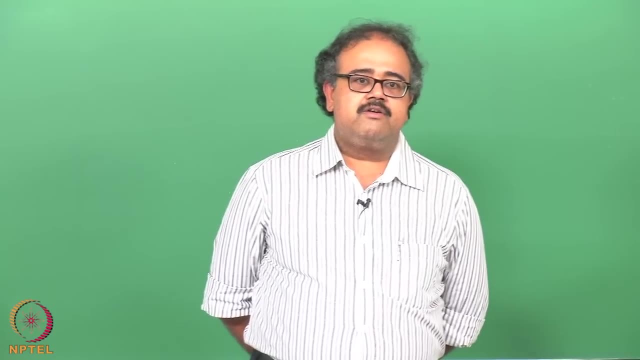 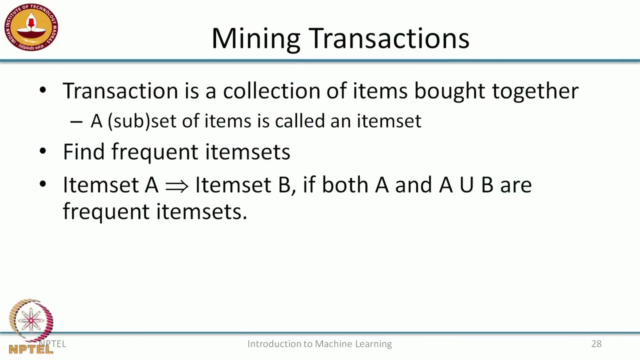 an item set in the association rule binding community, and so the first step that you have to do is find frequent item sets and you can conclude that item set A, if it is frequent, implies item set B if both A and A union B are frequent item sets. 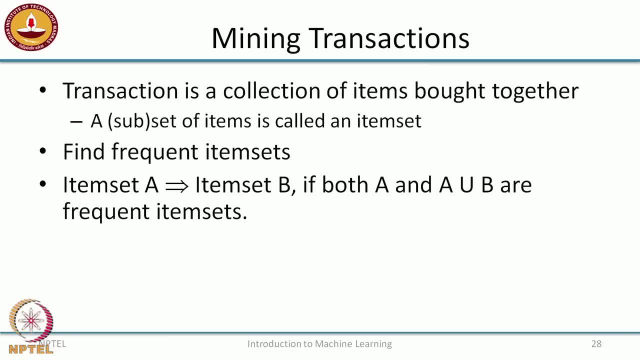 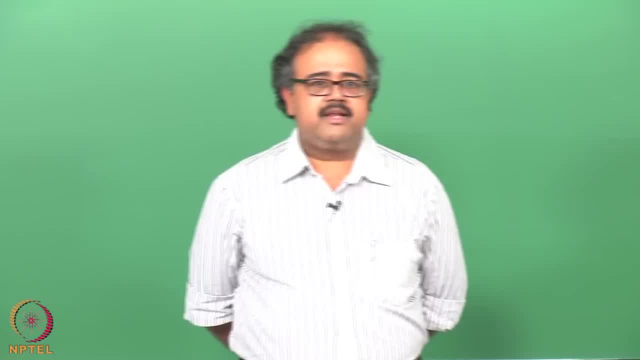 So A and B are subsets, so A union B is another subset. so if both A and A union B are frequent item sets, then you can say that item set A implies item set B and, like I mentioned earlier, so there are many applications here. so you could think of predicting co-occurrence of 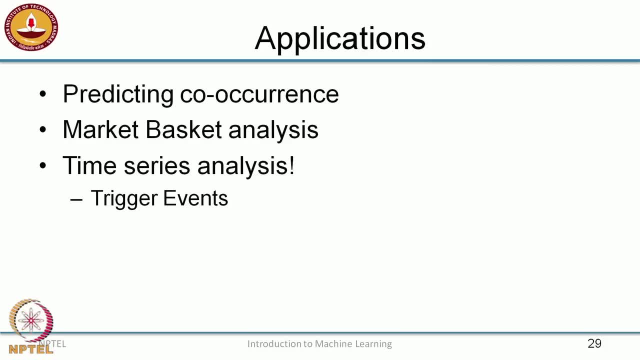 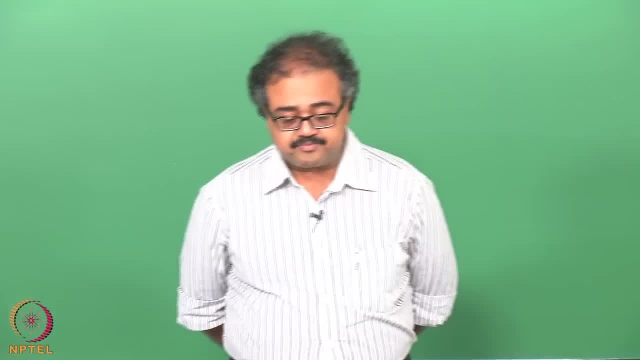 events and market basket analysis and time series analysis. like I mentioned earlier, you could think of trigger events or falls, causes of falls, and so on, so forth. So this brings us to the end of this module introducing unsupervised learning.